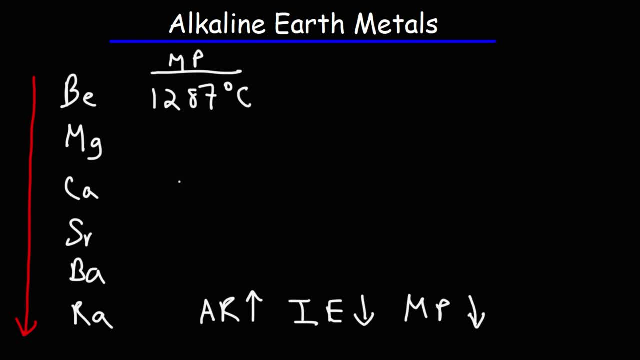 degrees Celsius. For calcium it's 842.. For strontium it's around it's between 770 and 780.. so it's like in this range. for barium it's 727 degrees celsius. so notice what's happening. 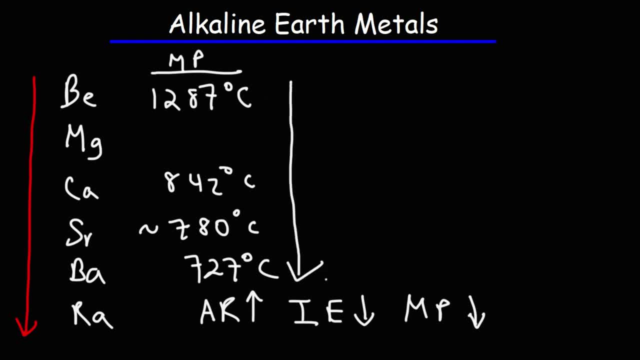 generally speaking, the melting point is decreasing as you go down. the melting point for magnesium is the lowest of the metals listed here. it's 650. so magnesium is the oddball for some reason. but generally speaking, as you go down the group, the melting point decreases. the ionization energy decreases but the atomic radius increases. 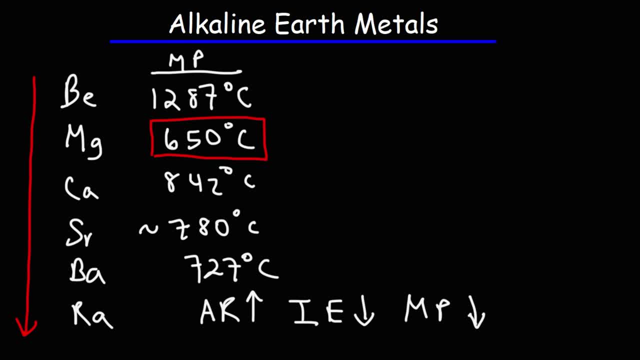 now, as you go down the group, the alkaline earth metals become more reactive, so the reactivity of these metals increases as you go down the group. so what this means is that so, since calcium is below magnesium, calcium is more reactive than magnesium and you can look up. 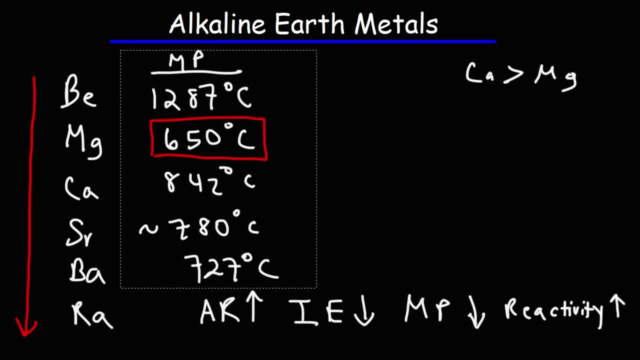 some youtube videos on the reactions of alkaline earth metals with water. you'll find that when you put magnesium in water at room temperature it reacts very slowly with water, so slow that you may not even notice any observable reaction. you might see a few bubbles calcium- it reacts faster with water than magnesium. you can observe the reaction. 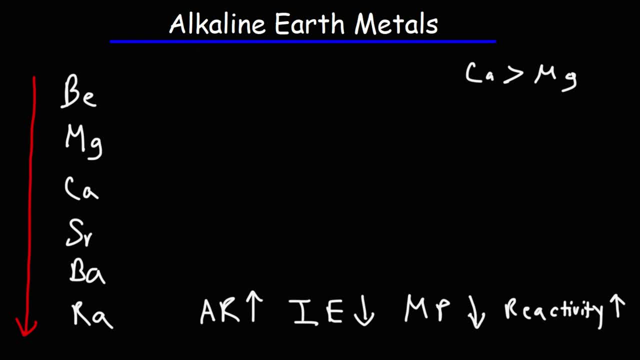 however, alkaline earth metals. they're less reactive than alkaline metals. alkaline metals, like lithium, sodium, potassium, they react vigorously with water, but the alkaline earth metals, they react slower than the alkaline metals. so alkaline earth metals are less reactive than alkaline metals. so this means that when you put magnesium in water at room temperature it reacts. 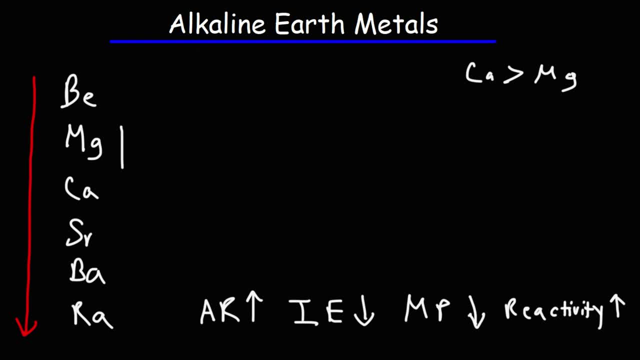 faster with water but, like alkaline metals, the reactivity increases as you go down. because the heavier elements they can easily give up their electrons, compared to the less heavier elements because the ionization energy is less as you go down, making it a lot easier to give. 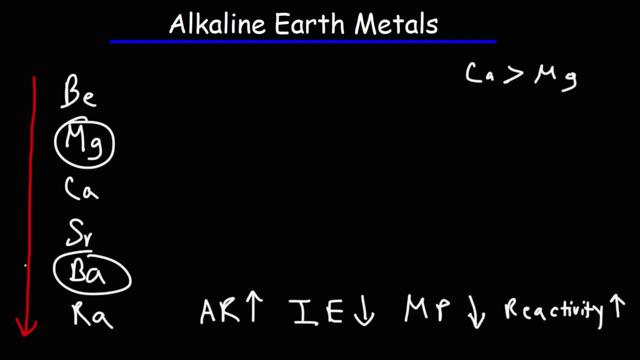 away the electrons making these metals more reactive with water. so when this happens, magnesium reacts with water. it will create magnesium hydroxide and hydrogen gas. so this process is slow at room temperature. however, if you boil the water- let's say if you put magnesium in boiling water- it will react faster. population gas solution. 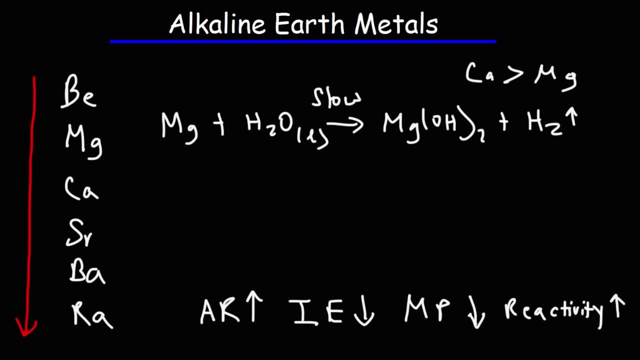 If you boil the water, let's say if you put magnesium in boiling water, it will react faster at higher temperatures. the yield r At higher temperatures, the yield magnesium dioxideイ with a oxide increases as a product rather than magnesium hydroxide. in fact, if you take 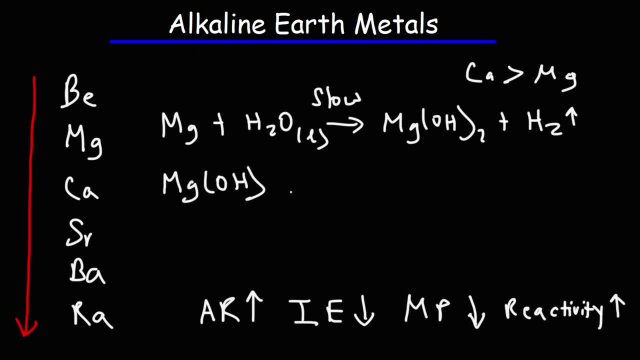 magnesium hydroxide, and if you apply heat to it you can drive off water from this compound. water can evaporate directly from magnesium hydroxide upon thermal decomposition. now the reaction between calcium and water is very similar to what we have here. calcium can react with liquid water at room temperature to create calcium hydroxide and hydrogen. 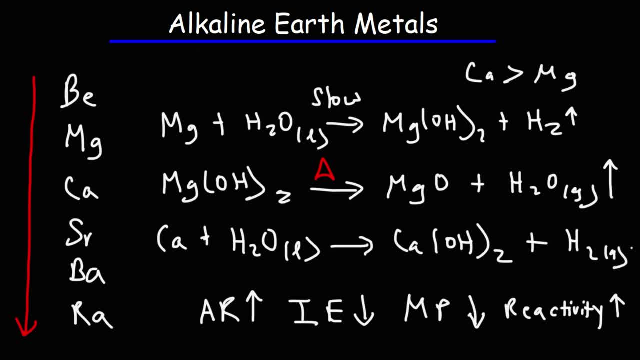 gas. so that's another gas evolution reaction. when you increase the temperature, you're going to drive the reaction to the right, favoring the release of gas in that reaction. now, alkali metals, because they like to give away electrons. they're reducing agents. they're strong reducing agents. 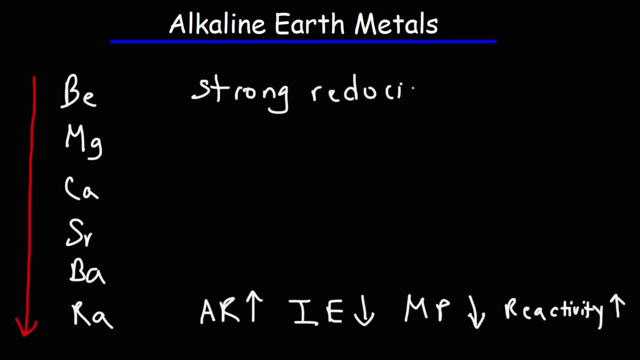 you. metals tend to be reducing agents, non-metals tend to be oxidizing agents. so oxidizing agents like oxygen, fluorine, chlorine- they like to take electrons, but reducing agents like to give away electrons. alkali metals are one of the strongest reducing agents after that.